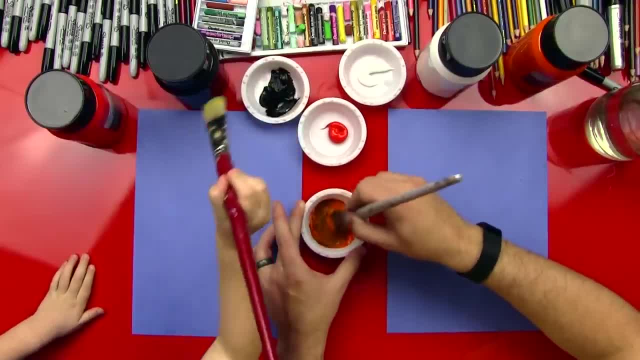 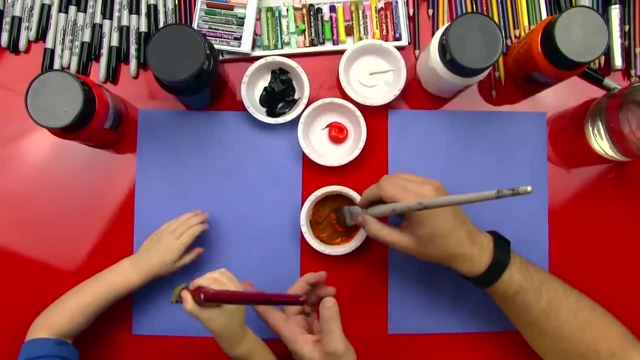 bit too, and you can help me mix. that sounds like a good idea and that's probably too much brown, but go ahead and put it in there and let's see what it looks like. okay, go ahead. or too much black? but go ahead, you mix it, you take a turn and mix. that isn't that awesome, does that look? 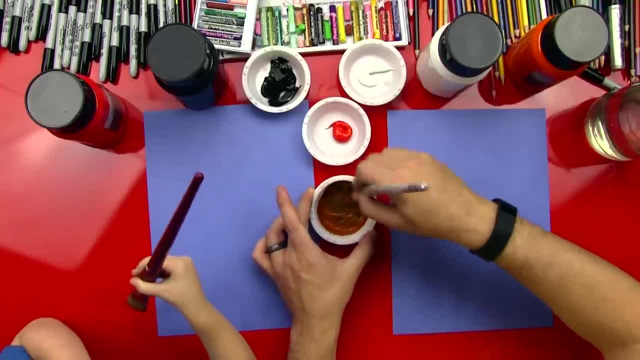 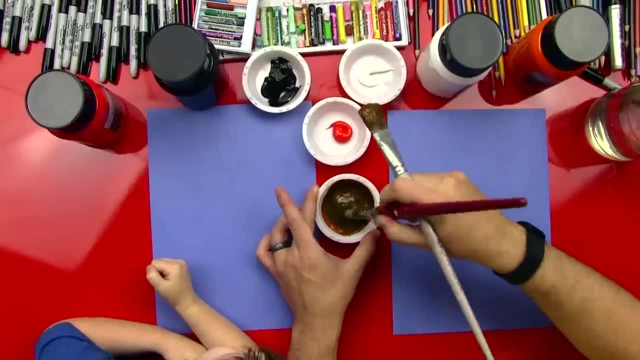 like brown now. yeah, we can put a little more orange in there. huh, let me see your paintbrush. i want to make sure we mix that black so that we don't. yeah, this is kind of a tough brush, huh. yeah, but you'll have fun with it. let's put a little more orange in there, huh. 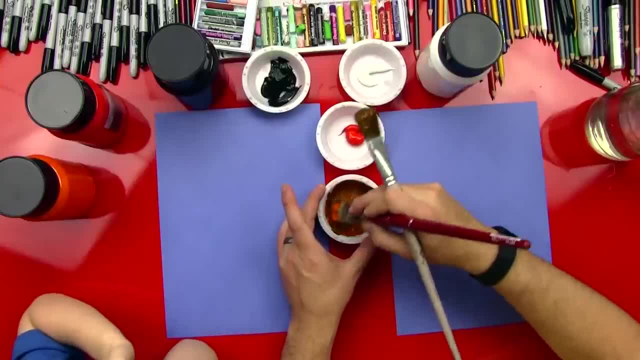 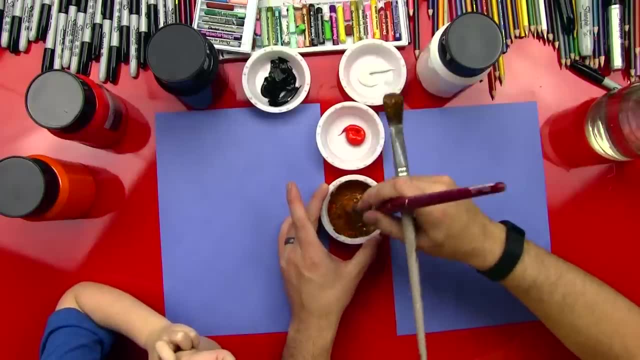 yeah, that sound like a good idea. yeah, all right, we got a nice brown, huh. okay, we're gonna do the tree first. okay, well, let me get some of this mixed up a little more. all right, so we're going to do the tree first. yeah, you hang on to that brush. 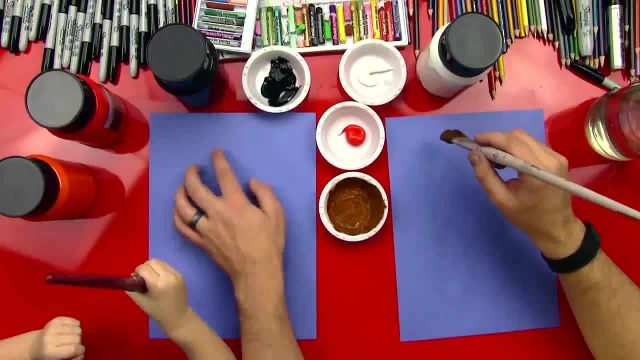 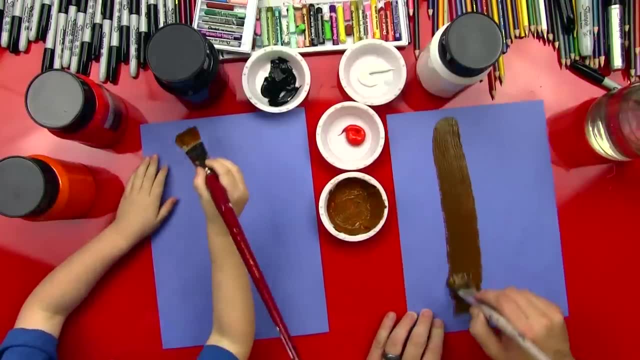 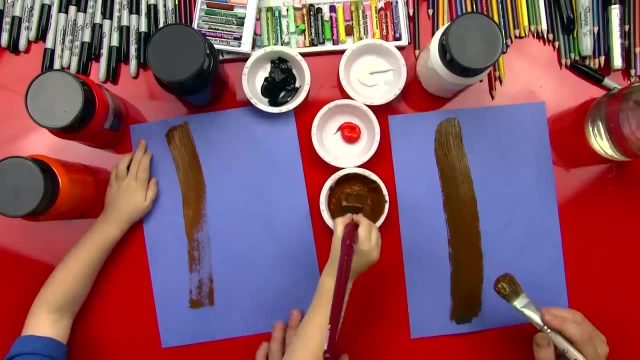 and then what we're going to do is we're going to do a line. we're going to start right here at the top of our paper and we're going to do a line that goes down: okay, okay, so go ahead and do that line. yes, perfect, you can flip over your brush. you have some more paint on the other side. 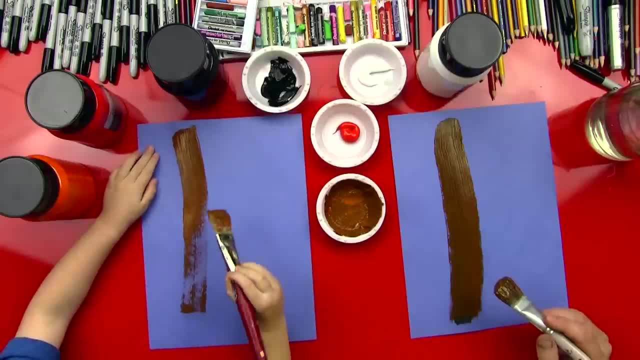 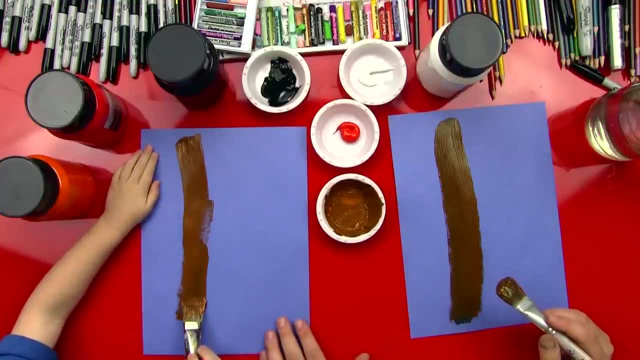 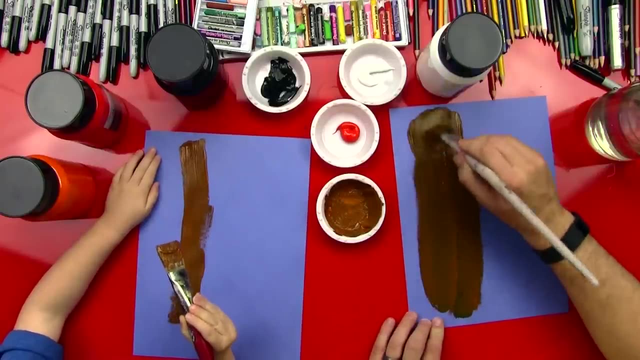 flip it this way. there you go, whoop, and then finish your line right there. finish that going all the way down. good job, chaos. now we're going to paint this side of our paper, okay, okay, can you do that? and i'm going to go ahead and paint on the counter. our art friends should always ask their parents if 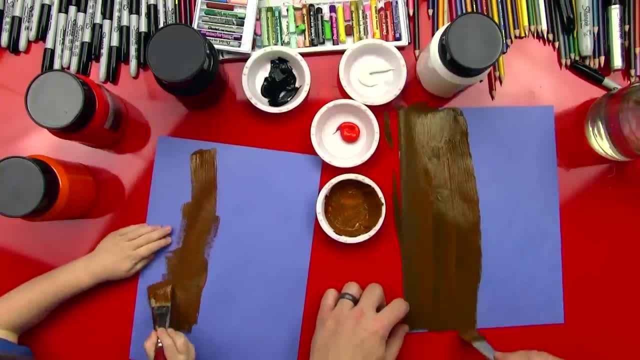 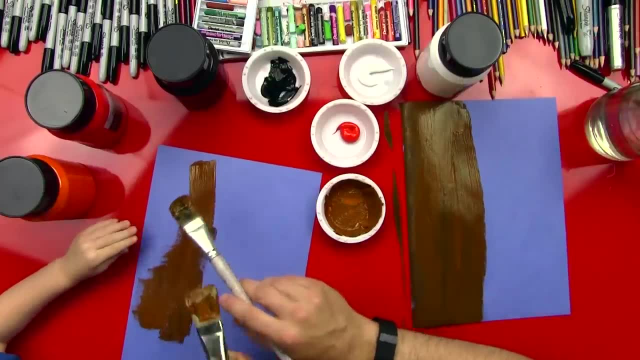 it's okay to paint on the counter or on the table. you don't want angry parents wondering why they're table is brown. huh, okay, use this. there's more paint on this brush, okay, and then i'll rinse this one out for you. yeah, that's okay on the. 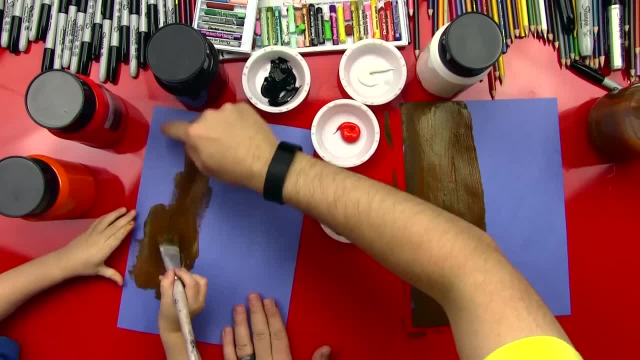 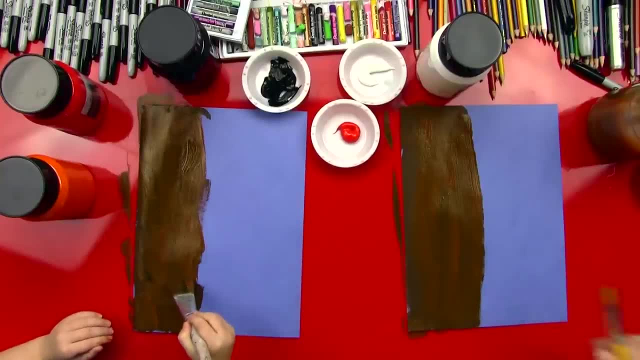 there we go, we can clean it up. okay, go ahead and paint all the way up there. good job, austin, you did it. okay, we got a little paint on your fingers. we could just wipe it off. huh, yeah, that's no problem. all right, little med, you ready to go? 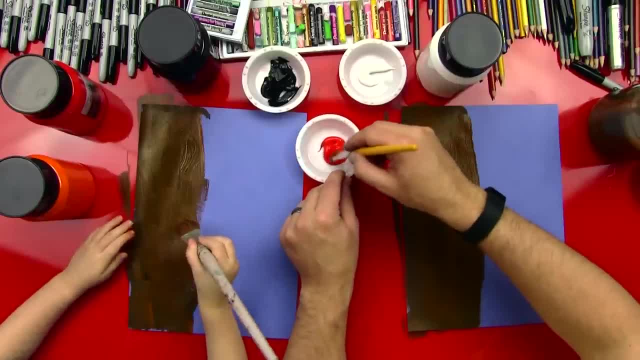 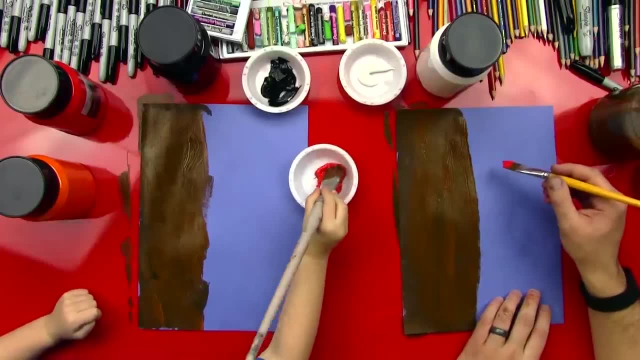 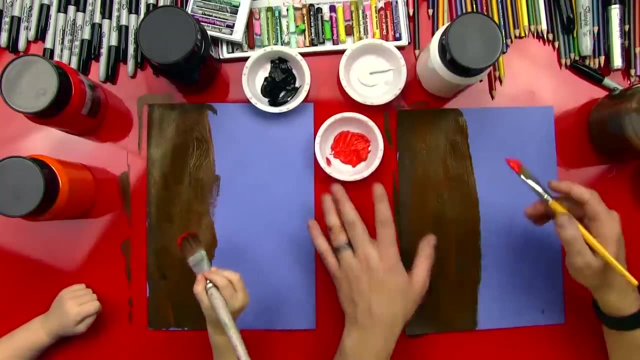 you ready for the our woodpecker's head? we're gonna get some red on our paintbrush, so get some red on that, get some red on your paintbrush and then watch dad. okay, okay, get a little more good. okay, now we're gonna do a little circle. it's gonna be a really small circle right here up. 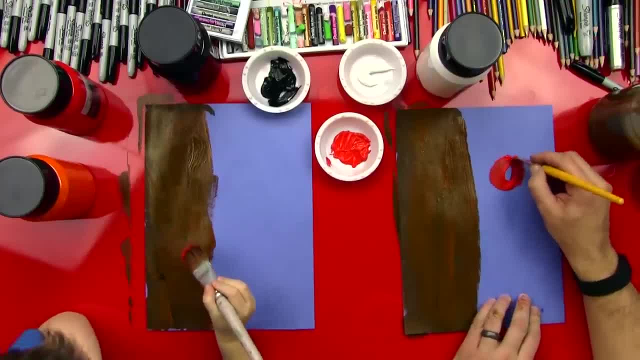 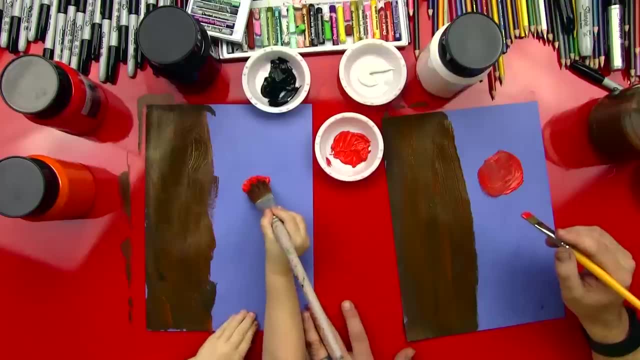 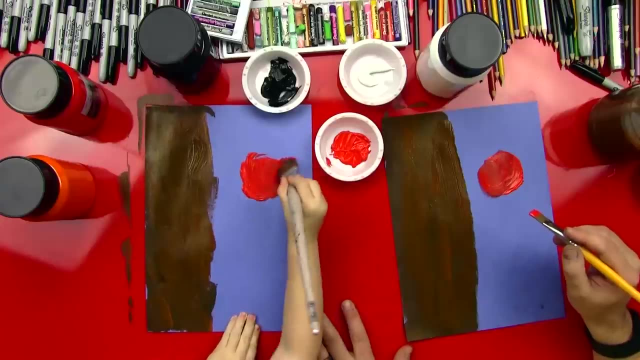 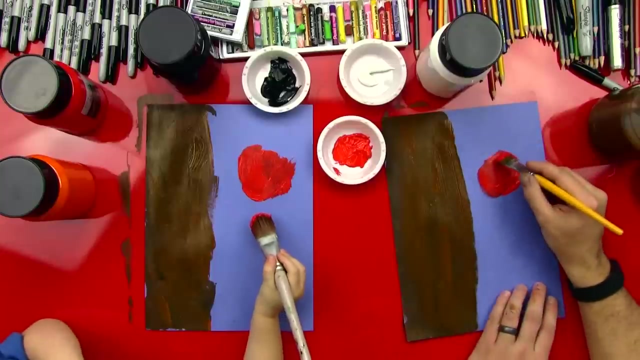 right there, watch this. there's a little circle. can you do a little circle like that right here, right here? yes, just a little one. you can do a little bigger. there we go, keep going, perfect. okay, now we're gonna put a little tail on his head. okay, we'll get a little more paint and we're gonna do a little line that comes up. let's do a little. 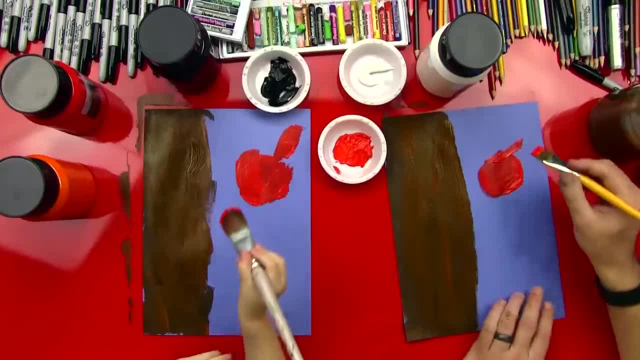 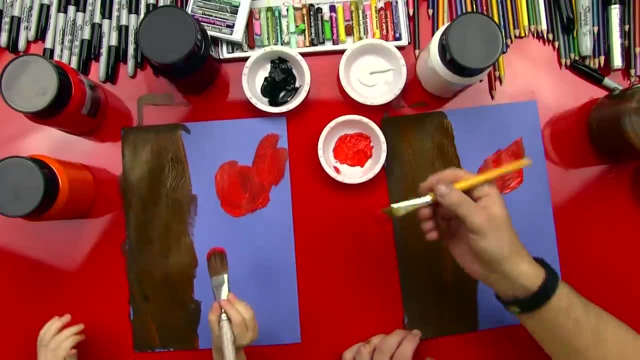 line right there. yeah, we're a big one, and then we're gonna come back down and that's gonna be for our woodpecker's head. okay, now we're gonna do a little circle like that right here up the back of his head. yes, good job, you did it. okay, now let's rinse this off because we're all done. 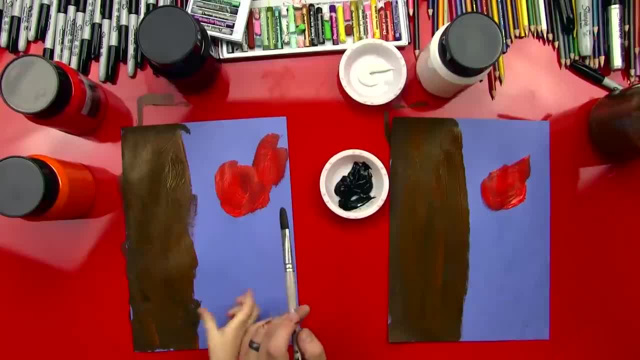 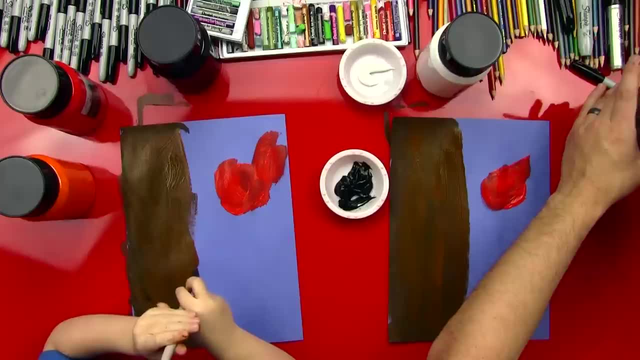 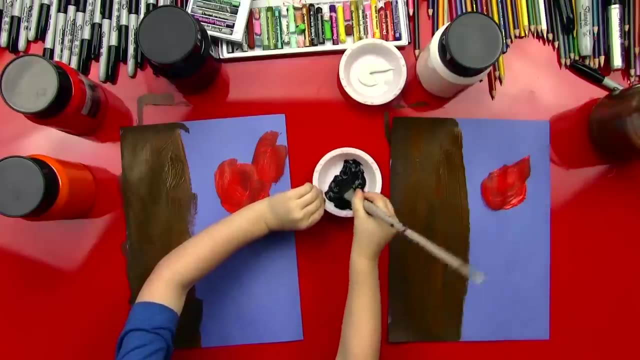 with the red, okay. okay, now we have a slightly smaller paintbrush because we're gonna do some little parts on our woodpecker, huh yeah, and get some black. so yes, get some black on your paintbrush. i'm still rinsing off mine. we're gonna do a little bit. we're gonna do a small little. 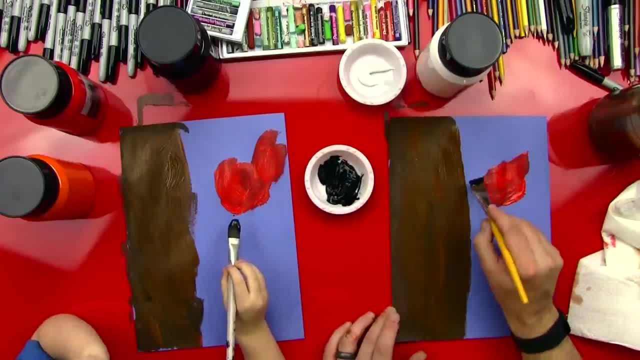 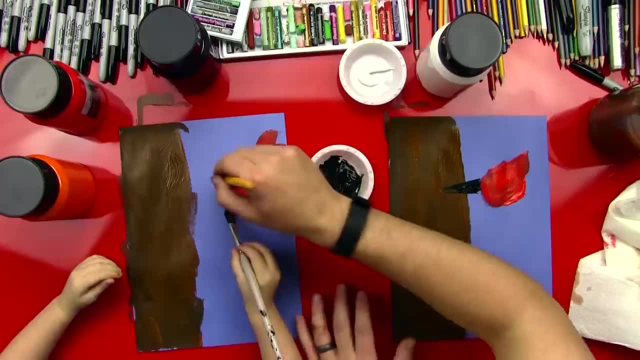 bit of paint on our woodpecker, and then we're gonna do a little bit of paint on our woodpecker, okay. so we're gonna do a little line. watch this. here we go from the side and again a small little v- like that you can do a little- go start in the head. okay, start there and then go out and then. 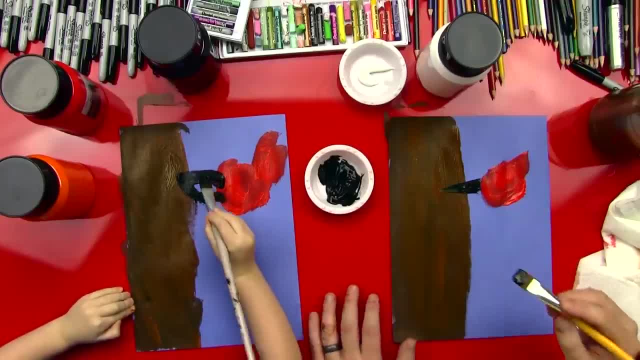 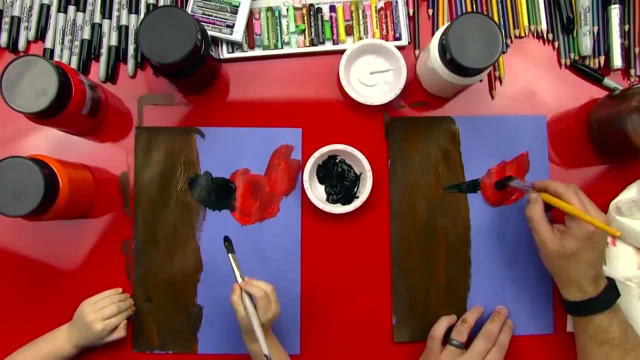 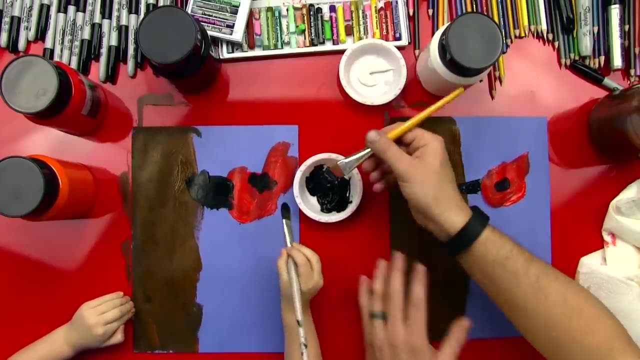 back in. good job, you did it and then paint it in. okay, now we're gonna do his eye. we do a little circle right there for his eye. good job, boss. all right, ready for his body. yeah, here we're gonna do a line that comes down from: 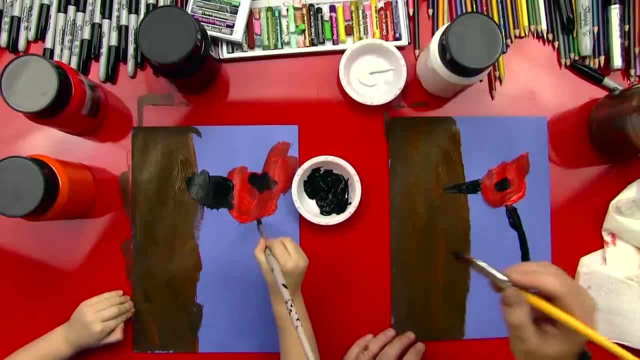 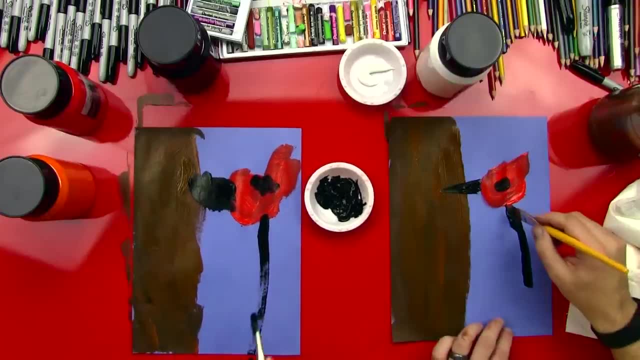 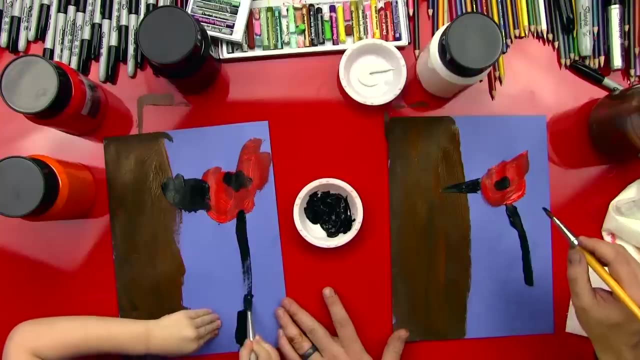 his body from his head. i mean, yep, start from his head and do a line down, hang on to the paper. there you go and then stop. good job, and then you want to get a little more. i like how long you made his body. good job. you're such a good painter, you made that line perfect. 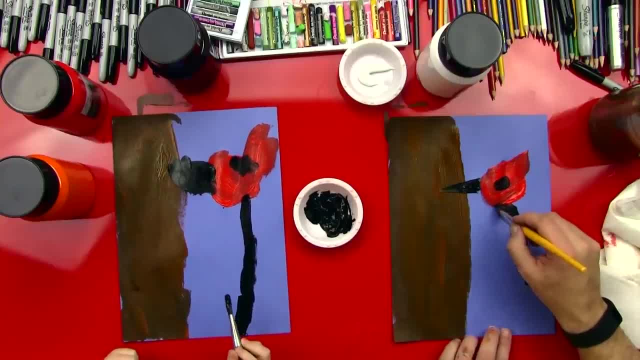 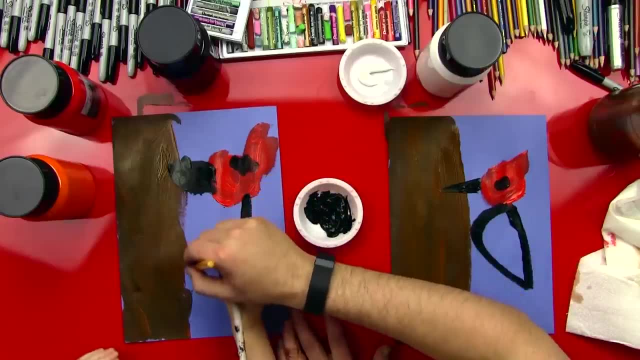 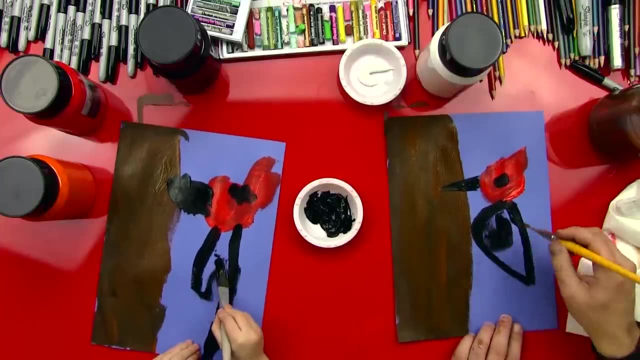 perfect, okay, now we're gonna do a big. it's almost like we're making a d backwards d, like that. you see that. so start right here and go out and then back in. out, yep, and then back in, yes, and then paint it in and paint that his body in. 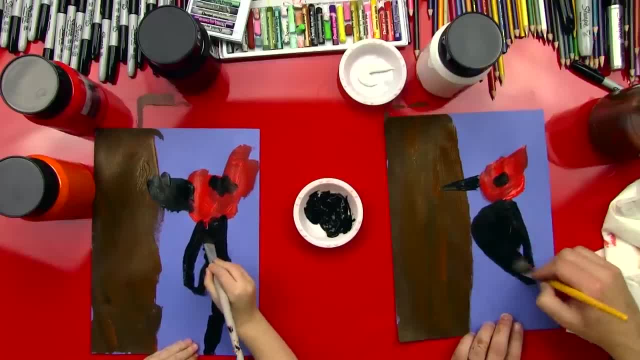 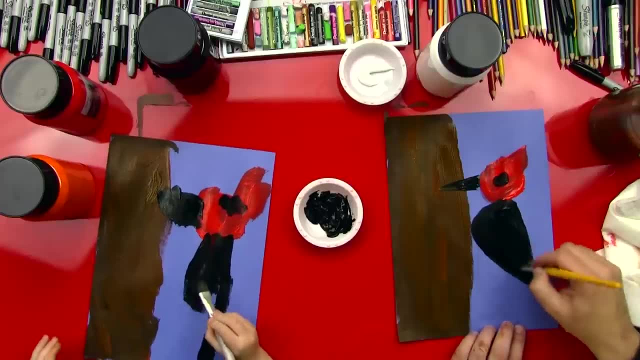 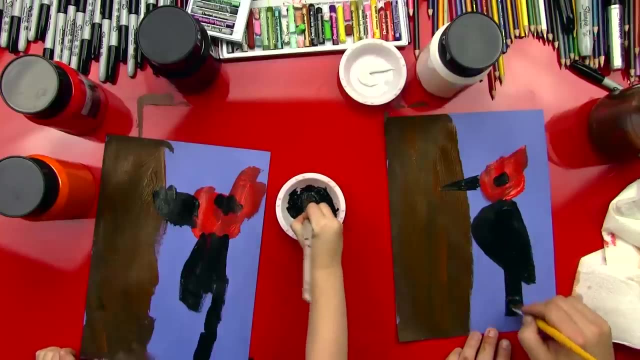 good job, all right. okay, now let's do a little bit of paint on our woodpecker. let's do his tail, so we do a little more and we could just do a line down for his tail. you need a lot, you need a lot and then just do it. that's probably a little too much. here we go, i'll. 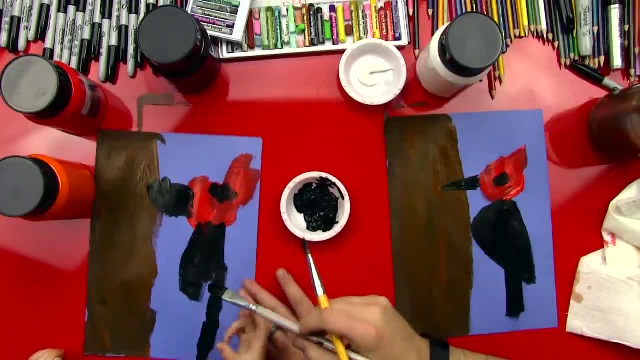 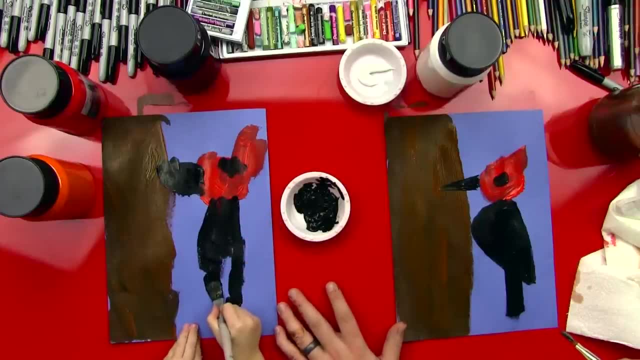 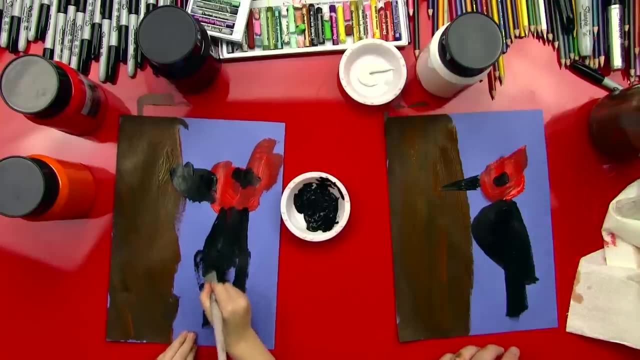 help you there. we go, get a little off there and then you can do a little line that comes down for his tail, yeah, and then come down and then stop. good job, okay, now we're gonna rinse this off and we're gonna get a little bit of white. all right, there you go. awesome now. 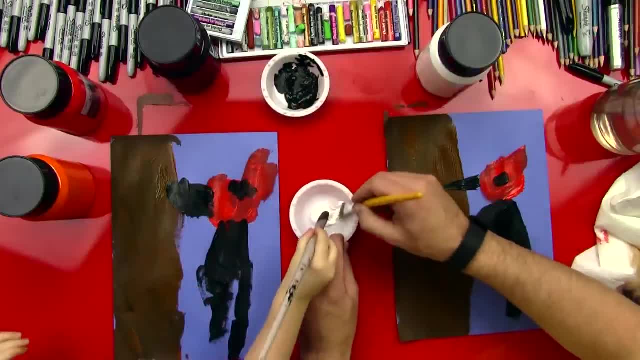 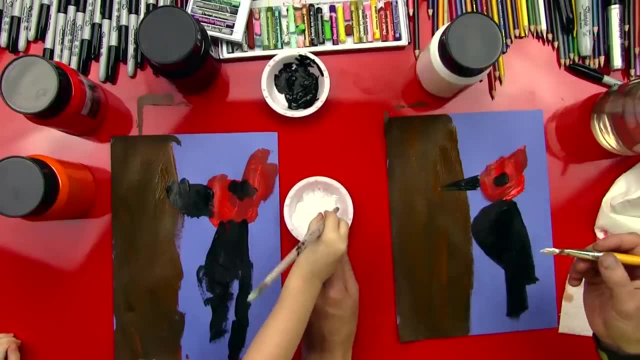 we're gonna get a little bit of white and we're gonna do his belly, because they have little white marks on their neck. okay, you got a little white on there, we're gonna do. this is a cool step we're going to come up to here and we're 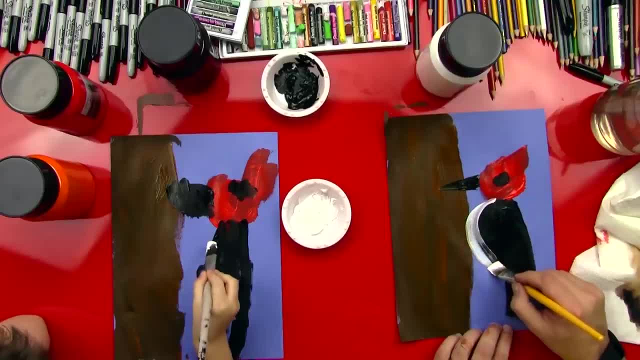 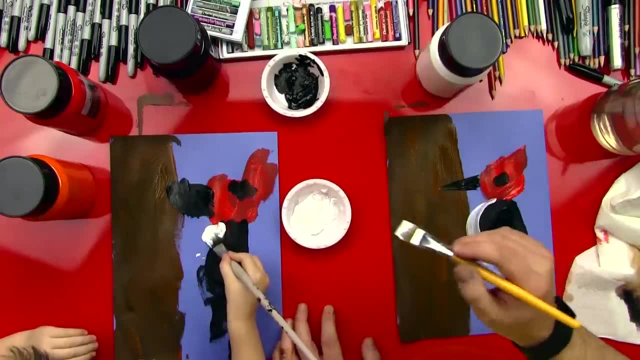 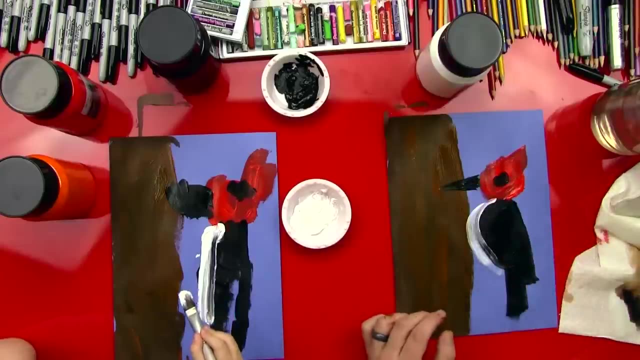 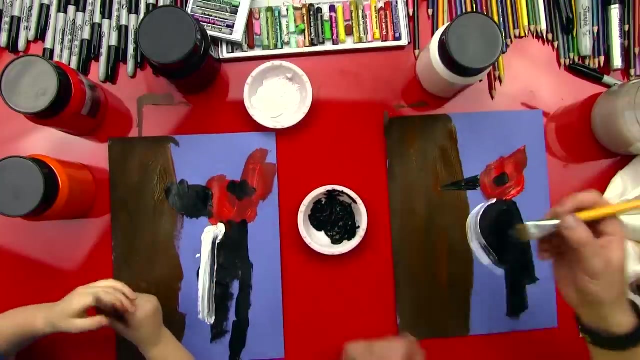 gonna do a line on his belly like this: do you start right here and then go all the way down to his belly? sorry, that's okay, and then and then stop. good job, you did it. okay. now let's rinse this off. almost okay. now we're gonna do a little more black and this is gonna be for his legs, okay. 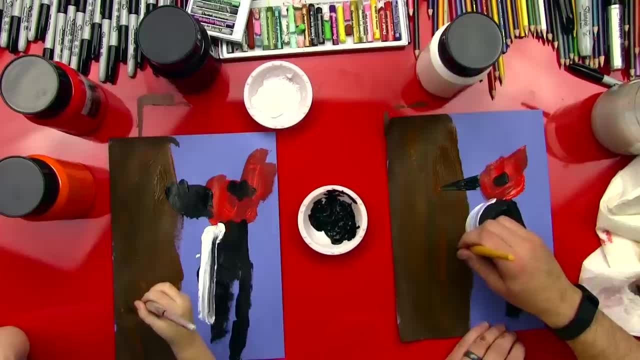 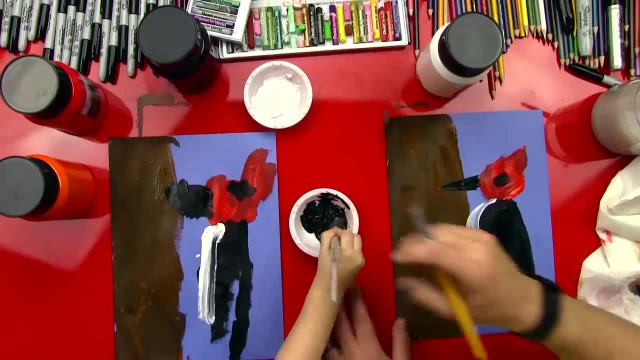 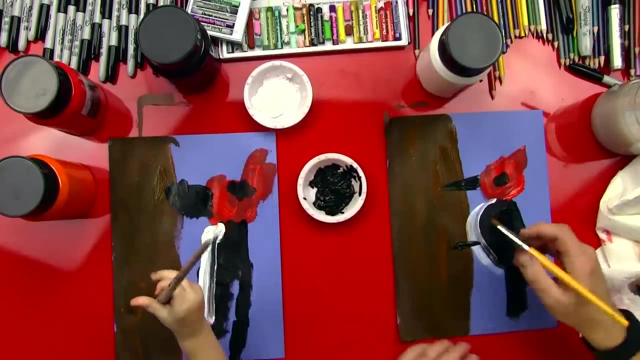 we're gonna do one line that comes out from his belly. you see this: get a little black on your paintbrush. good job, that's awesome. i'll help you a little bit. here we go. okay, now, awesome, watch this. look, you see this little line. yeah, do a line that goes out from his belly and connects to the tree, right? 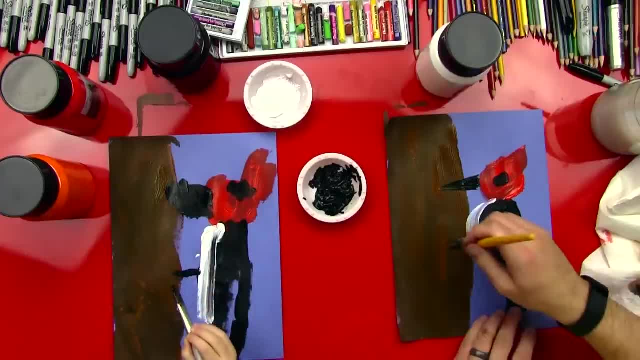 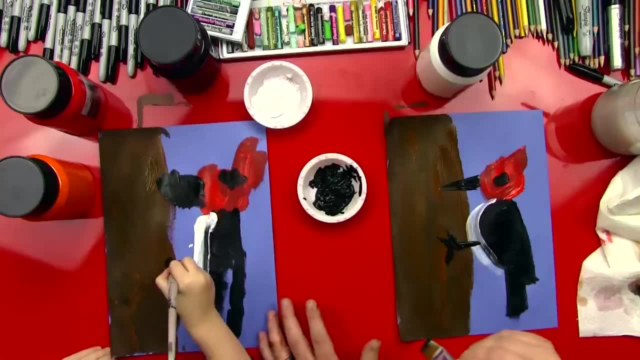 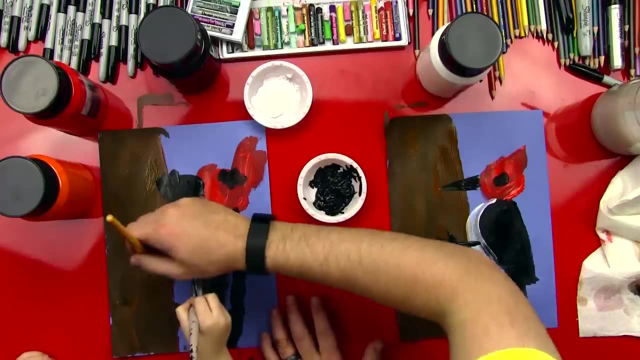 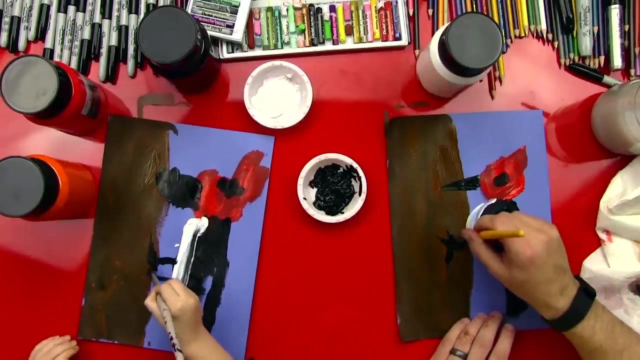 there, just a little one, and then you can stop, and you can do one, two, three for his little, his little feet, his little toes. okay, do another one, do another line, that goes out there. yeah, you could do another leg too. i like that. i'll put another leg in there too. 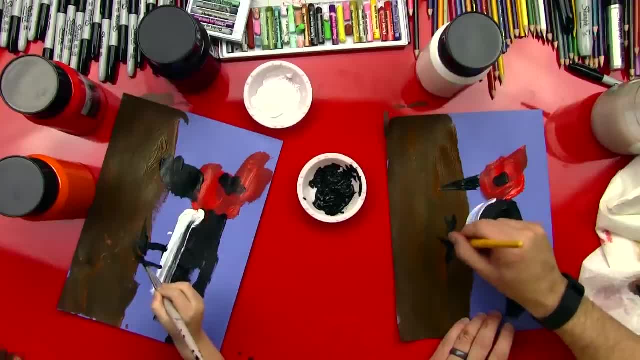 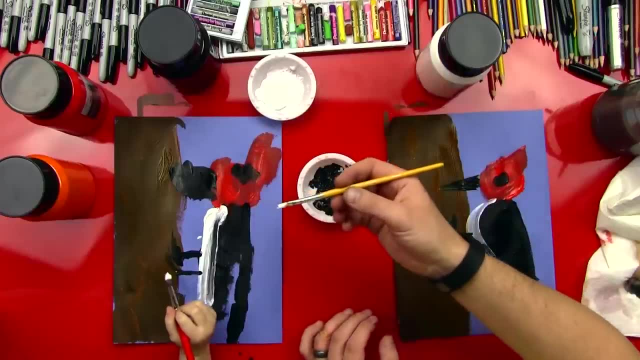 you got it awesome. you did the legs. you know what we could do. one last thing: all right, austin, we just got. we got a little paintbrush or got a little bit of white and we're gonna put a little dot on his eye. and put a little dot on his eye, yeah, 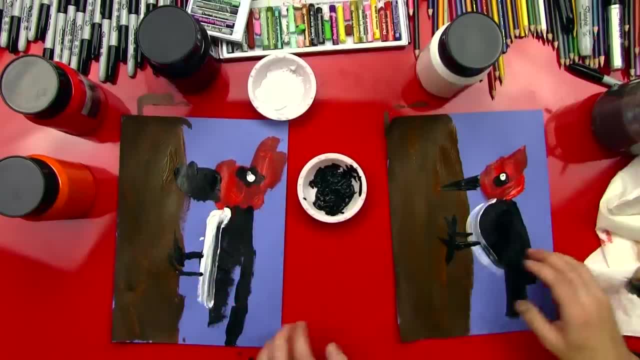 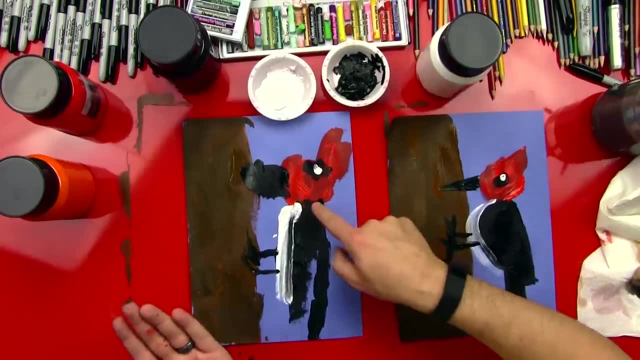 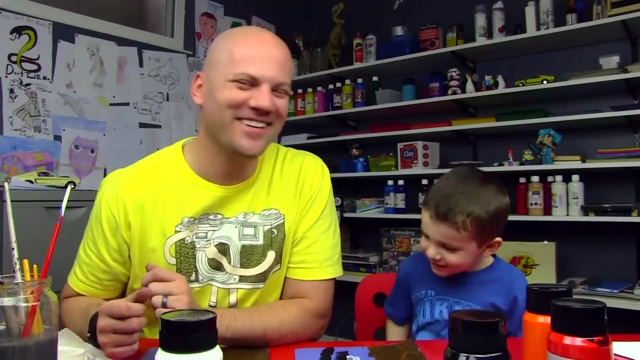 perfect, you did it. you finish. your woodpecker looks so awesome. did you have fun? yeah, you promise, give me five. he looks really cool. what should we name him? uh, woodpecker, woodpecker, how about woody? no, no, that's okay, we'll wipe it off. it'll all clean up. it cleans up after we use soap. 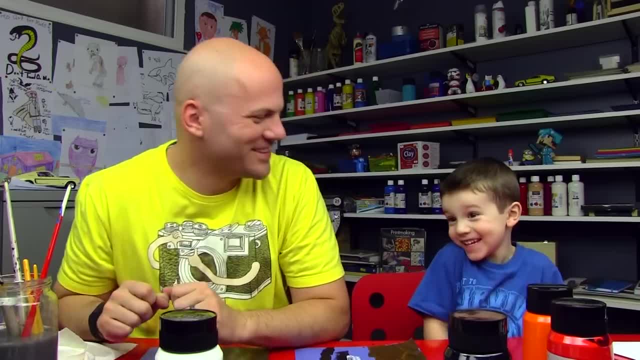 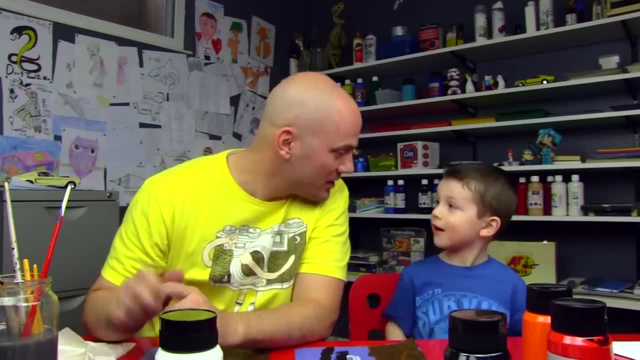 and stuff. did you have fun, you promise? we hope you guys had fun painting your woodpecker's with us. remember, this is a fun activity to do with your really young artists. huh, this is your three, right? yeah, this is a great activity for five and under, probably. yeah, yeah, should we say goodbye to our art friends and we'll see? 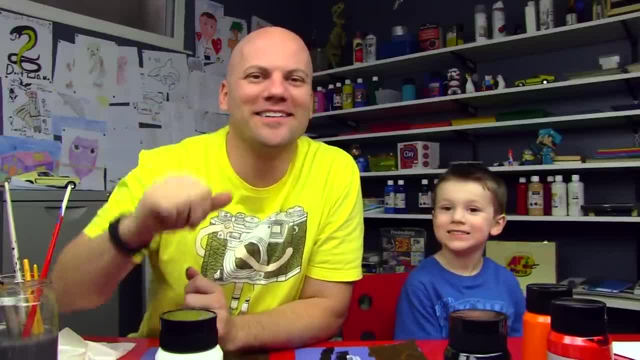 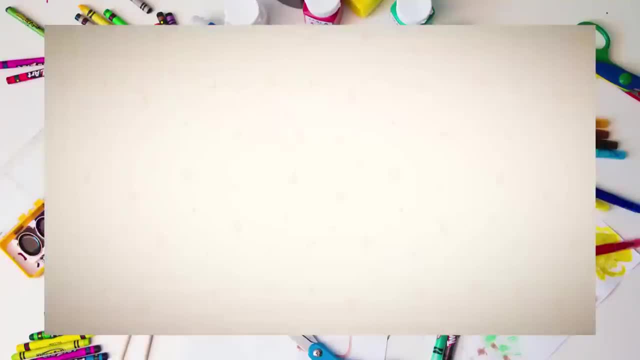 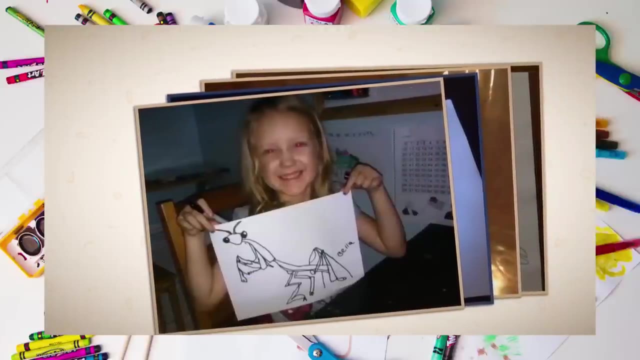 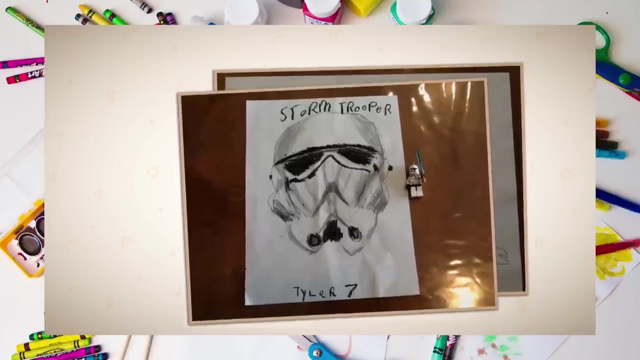 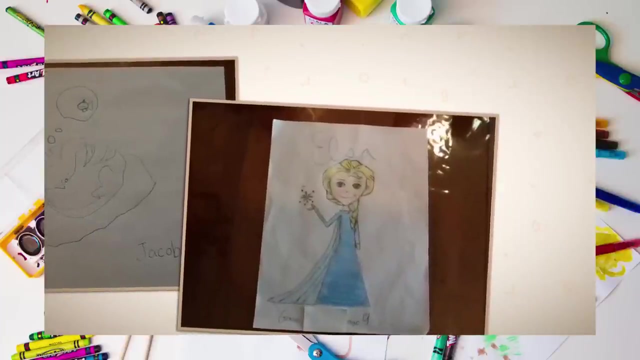 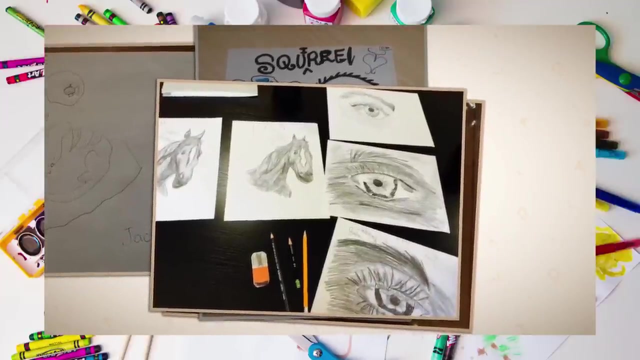 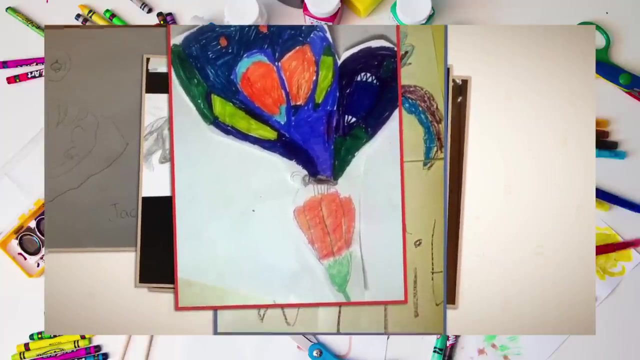 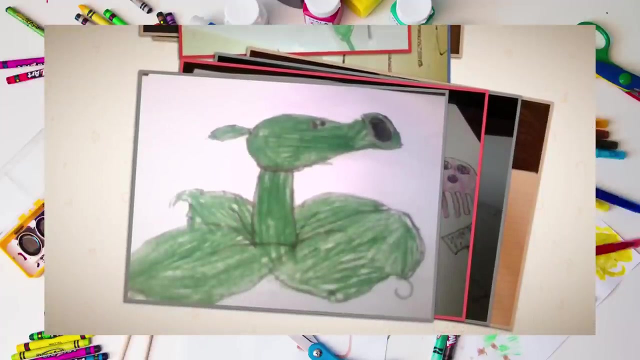 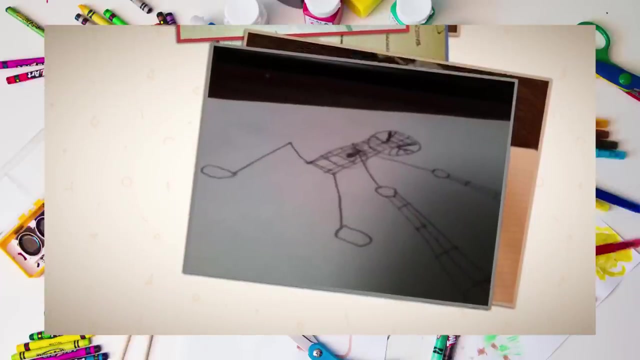 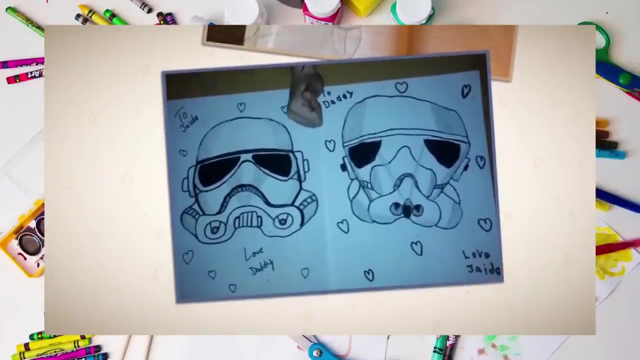 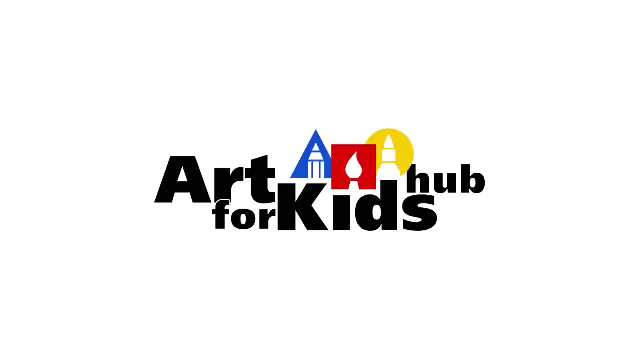 friends, see you later. our friends, goodbye. you're gonna wave you. wave you guys, you got wave you you.